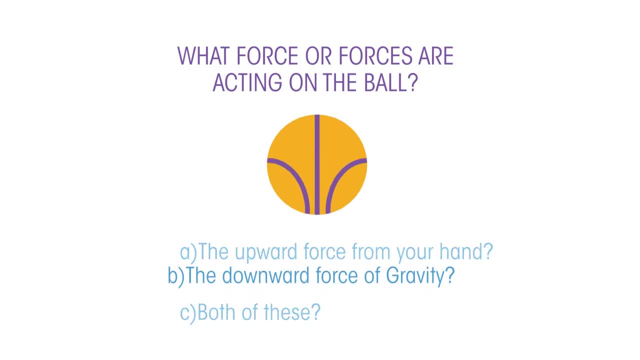 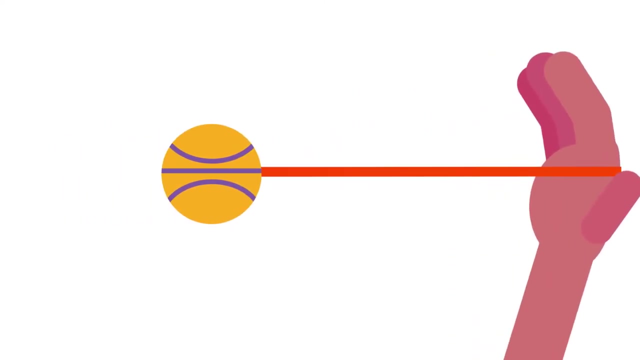 The answer is just the downward force of gravity, which gradually slows the ball, stops it, then brings it back down, making it fall faster and faster. The unbalanced force here causes the ball to change its velocity. Now look at this ball, thrown sideways but with elastic attached. The force on the ball must be. 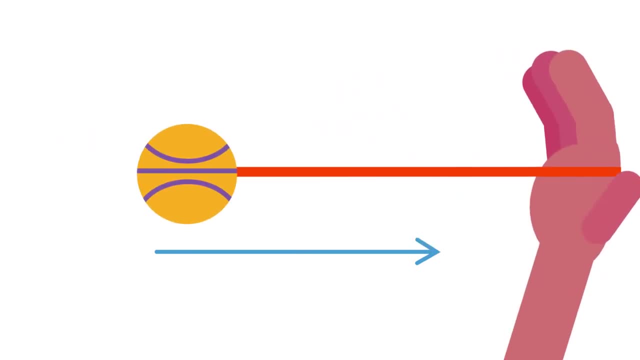 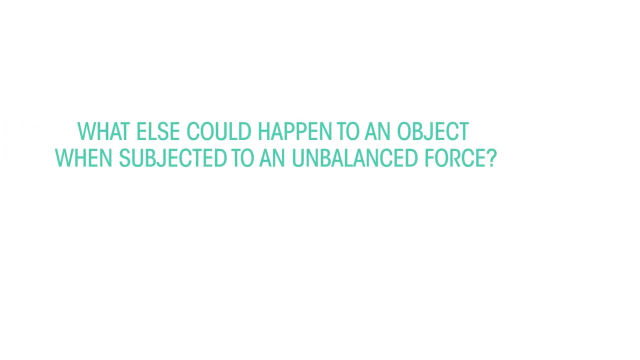 towards the hand, caused by the piece of elastic, which slows it down and then brings it back to the hand. This is just like the ball thrown upwards, except that it's the force from piece of elastic that slows the ball and then brings it back. What else could happen to an object when? 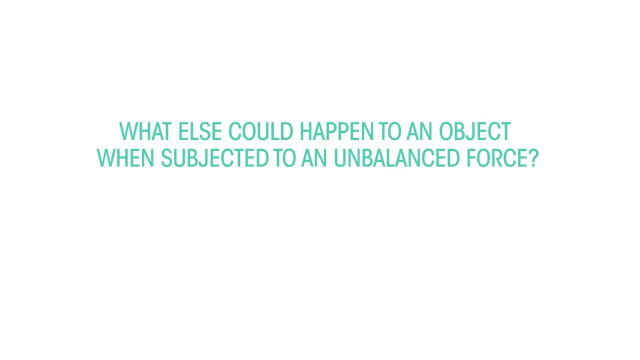 subjected to an unbalanced force. When forcing the ball to the side, the force is forced to the side. This is the force that is being forced to the side. When forces are unbalanced, objects can speed up, slow down, like the. 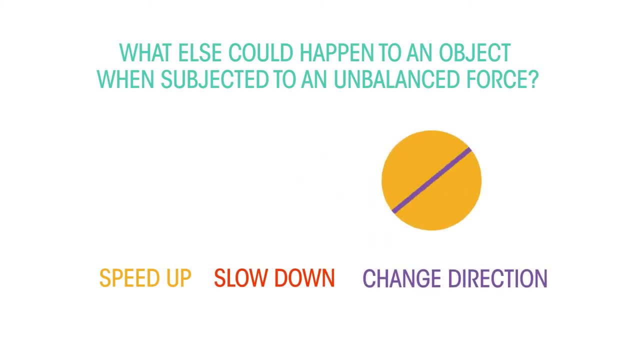 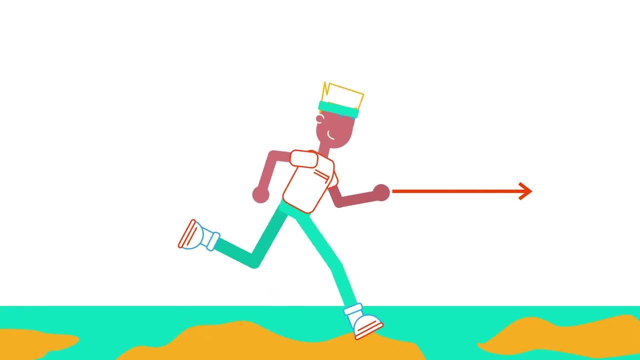 thrown ball but also change direction. Think of trying to change your direction on a muddy football field. Normally you dig your boot into the ground to provide the force to change your direction, But in the mud you just carry on in the same direction and you call it a skid. The larger the mass of an 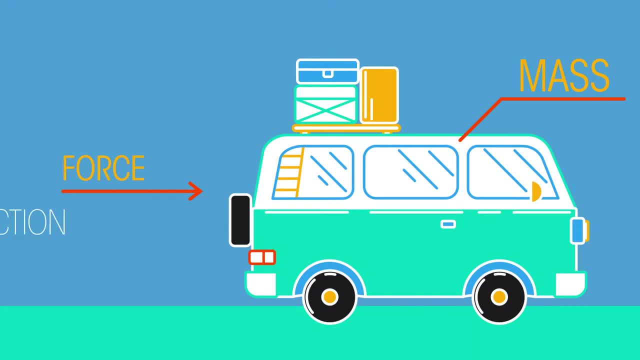 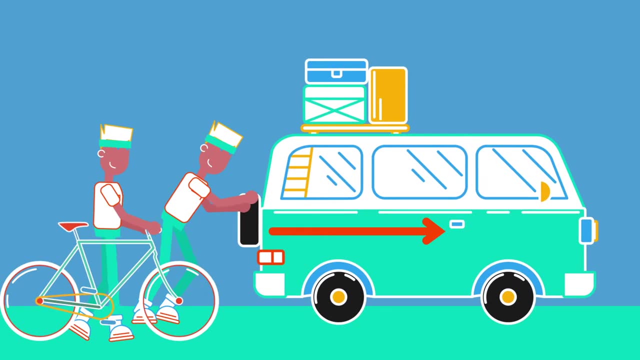 object, the larger is the force. This is called a skid. The larger the mass of an object, the larger is the force needed to change the direction or its speed. Think of trying to push a car compared with a bicycle. Also, the faster you want something to get moving, the bigger the force. 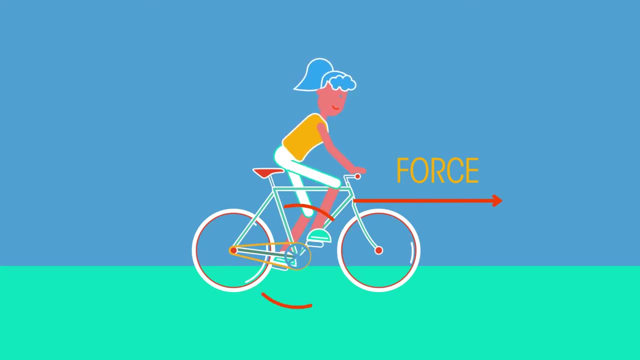 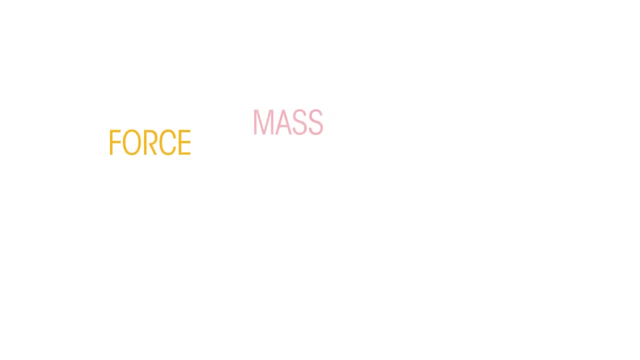 needed. Think of pedalling a bike: The harder you push, the quicker you get going. The relationship between force, mass and acceleration is known as Newton's second law, which means that you pull a car. the more you push, the faster you can get going. It consists of one-sixth of a second. 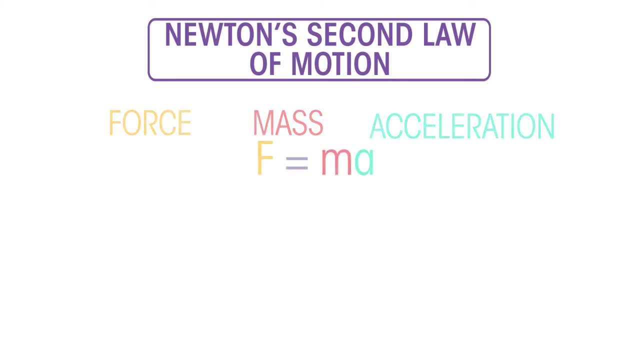 The force needs to change the direction or its speed. Think of trying to push a car compared with a bicycle law of motion. It can be summarized in this equation: Resultant force equals mass times acceleration. When force is measured in Newtons, mass is measured in: